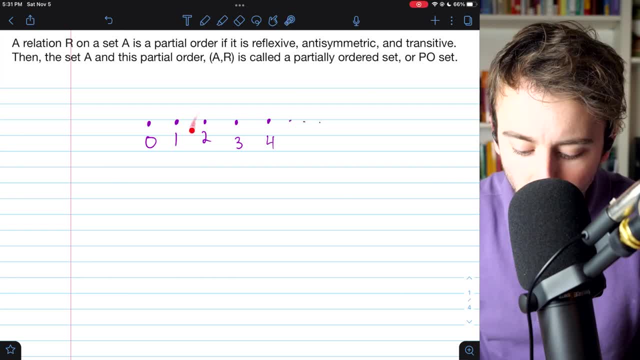 and, as far as we want, If you pick any two non-negative integers, we could certainly order them based on which is less than the other, which one is further along in the number line, But an ordering on elements of a set does not need to be this strict. We don't have to have every pair of elements. 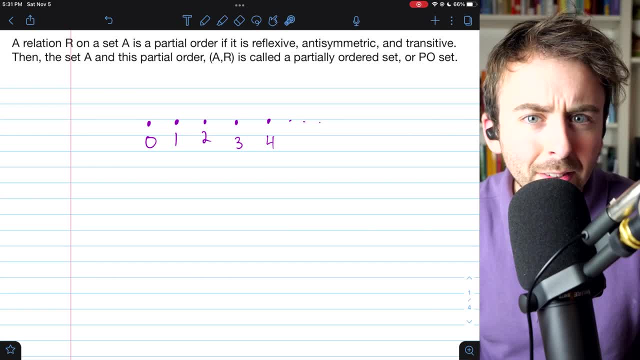 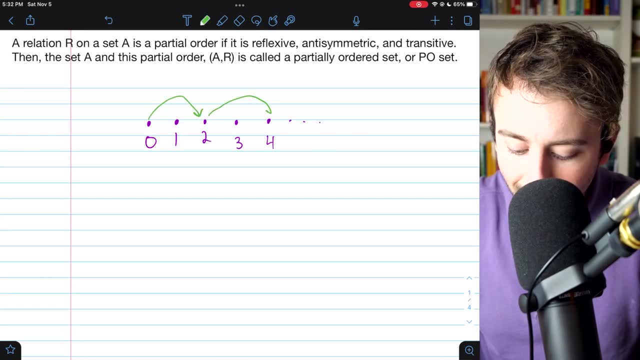 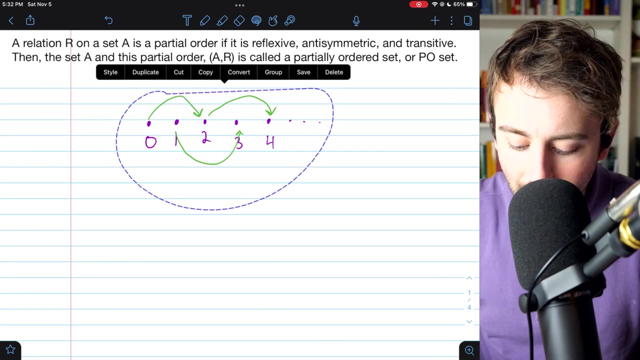 in some order. We could be a little bit less strict, and that's where partial orders come in. A partial order might only relate certain elements of a set. Not all elements necessarily have some relation to each other. Here is the definition first. 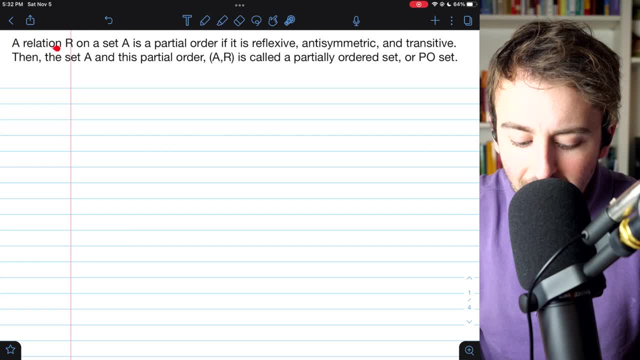 beginning with the definition of partial order. A relation R on a set A is a partial order. if it is a reflexive relation, an antisymmetric relation and transitive, Then if we take that set A along with the partial order R, this is called a partially ordered set or 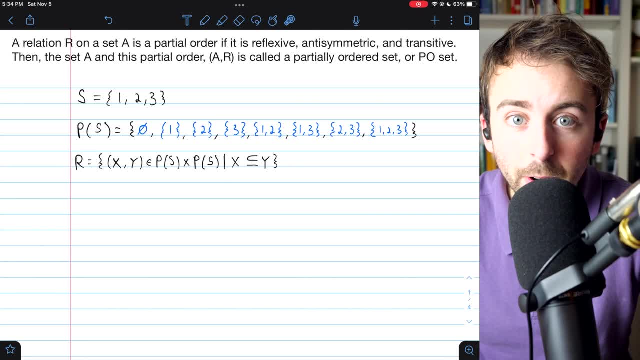 a poset, An example of a poset from set theory. let's say S is the set containing 1,, 2, and 3.. Then consider the power set of S. This is a set that we'll actually have our relation on. 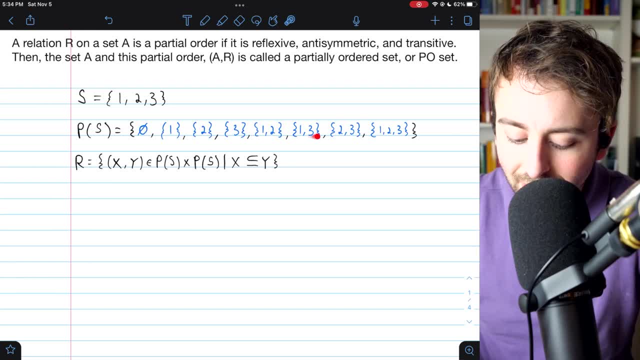 The power set, of course, is just the set of all subsets of the original set S. So this contains things like the empty set, the set containing 1 and 2, the set S itself, all subsets of S. Then 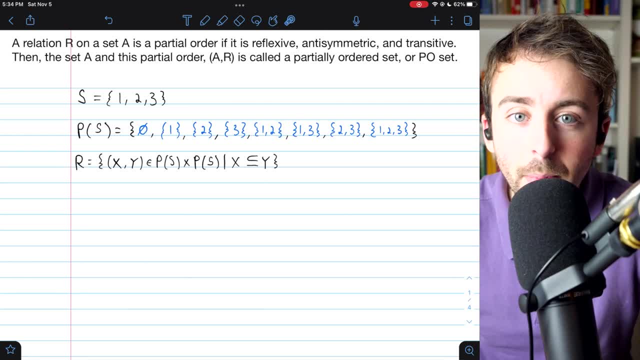 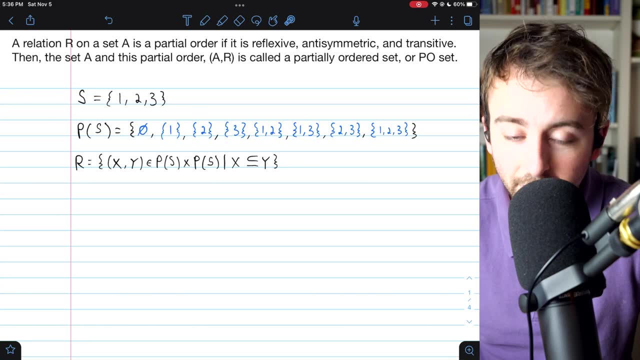 our relation r. our partial order on the power set is going to be the subset relation. I can just say that the relation is the subset relation. but let's just take a close look at r. Notice that it is the set of ordered pairs x- y, where x and y are both from the power set of s, so x and y are both. 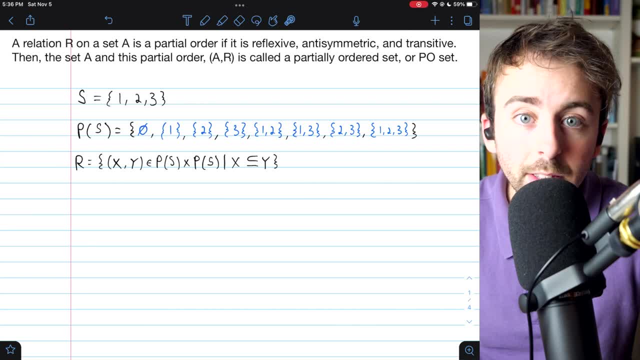 subsets of s, And we'll say that two elements, x and y, relate to each other, and thus the ordered pair x- y is in our relation. if x is a subset of y, Then the power set of s together with this. 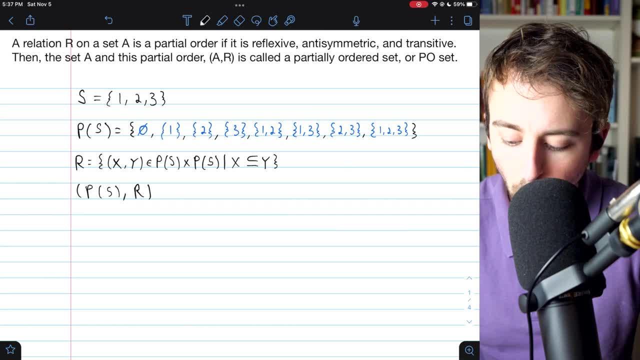 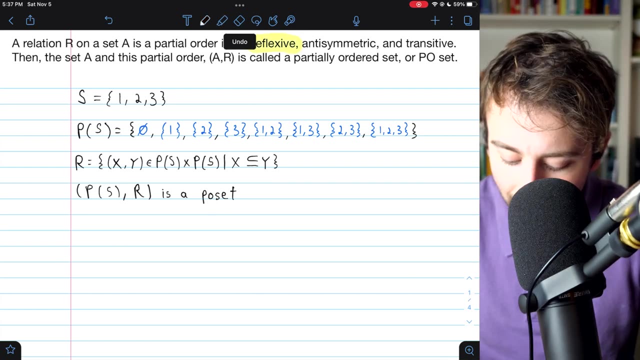 relation r forms a partially ordered set or poset. Now, why is it a partially ordered set? Well, we've got our set. p of s. It has been partially ordered because our subset relation is reflexive, since every set is certainly a subset of itself. 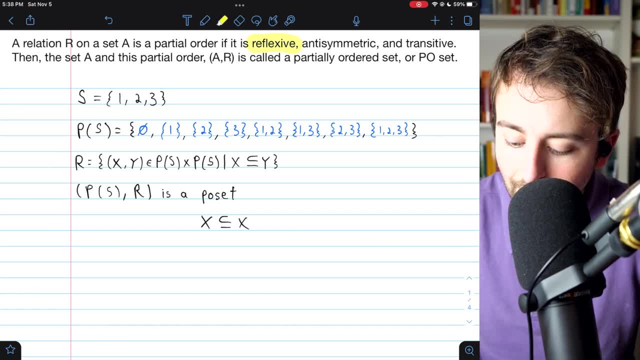 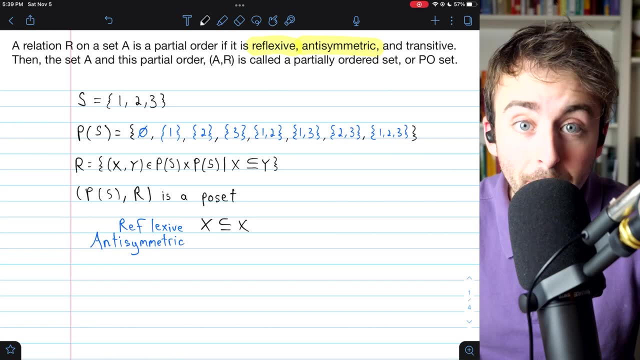 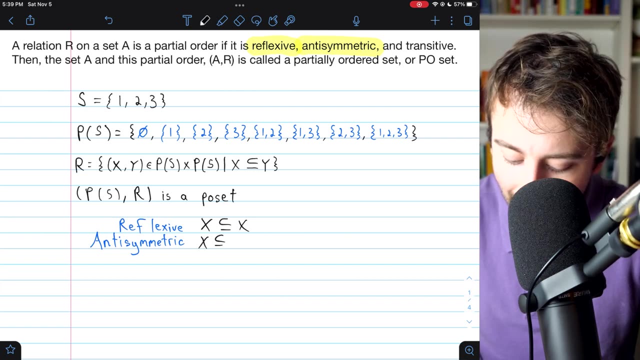 so it's reflexive. Also, the subset relation is anti-symmetric. A relation being anti-symmetric means that no distinct elements relate symmetrically, so no distinct elements relate in both directions. Said another way, this means that if x relates to y and y relates to x, then it must be the case. 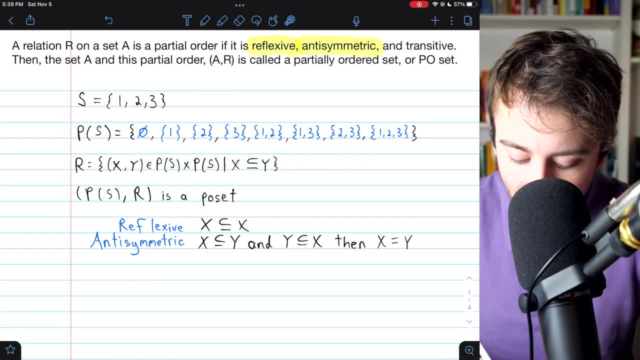 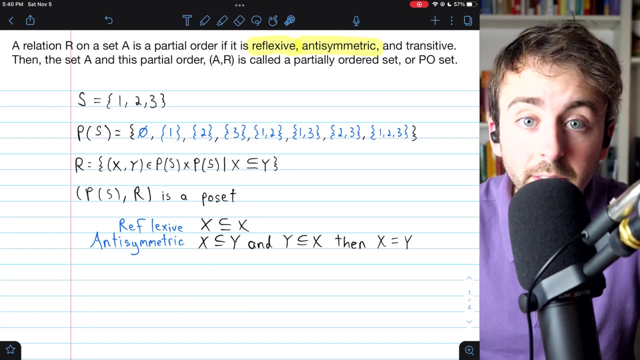 that x is equal to y. Again, this is because anti-symmetry means that no two distinct elements relate symmetrically. so if we have two elements that do relate symmetrically, well, they must not be distinct. They must in fact be equal. This is of course true of the subset relation. 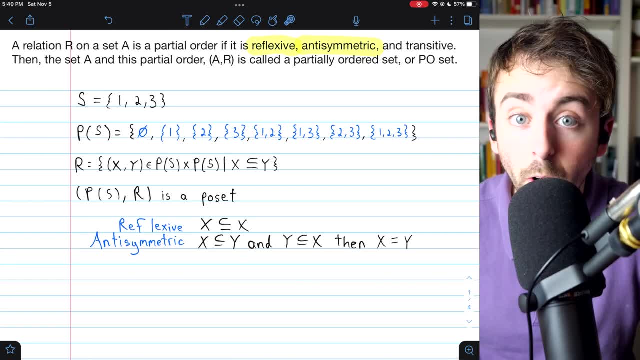 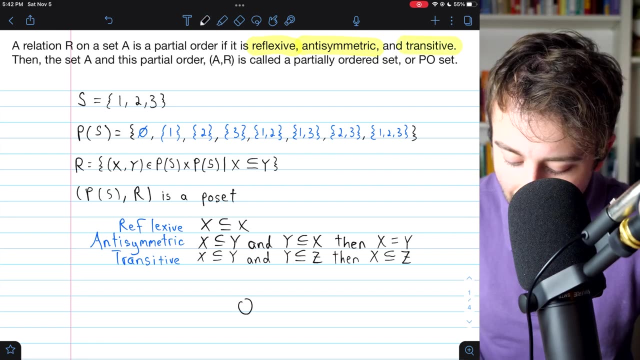 This is precisely how we typically prove that two sets are equal. If one's a subset of the other- and that's also true in the other direction- then the sets are equal. So classic example of an anti-symmetric relation. And of course the subset relation is transitive If x is an anti-symmetric relation. 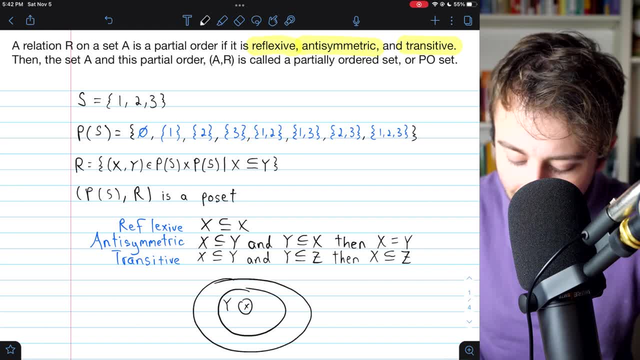 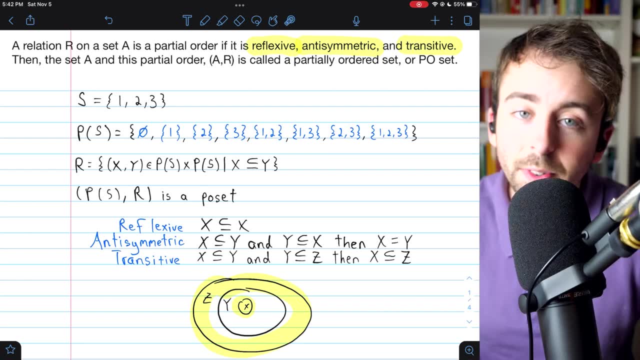 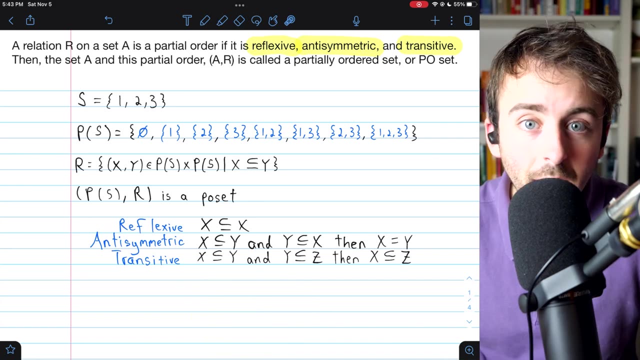 if x is a subset of y and y is a subset of z, then clearly x is also contained in z, and so, indeed, x is a subset of z, So subset satisfies transitivity. So that's what makes this a partial order and thus a partially ordered set. It's got a lot of nice order-type. 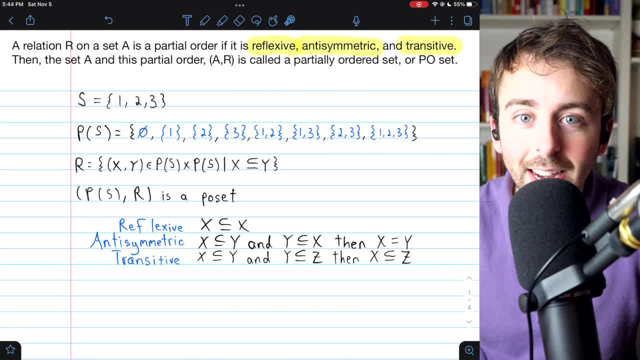 properties. You can travel from one element to the next via transitivity. X is a subset of, y is a subset of z, So x is a subset of z, And if two distinct elements relate to each other, they can't. 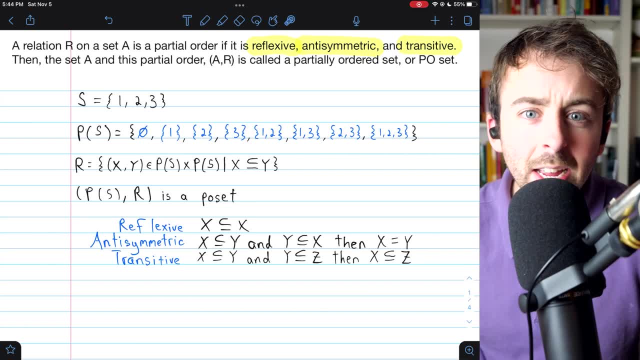 relate in the other direction. That's pretty important for an order, But it's a partial order because it's not required that all elements of the set relate to each other in some way. For example, if we consider the set containing 1 and 3, as well as the set 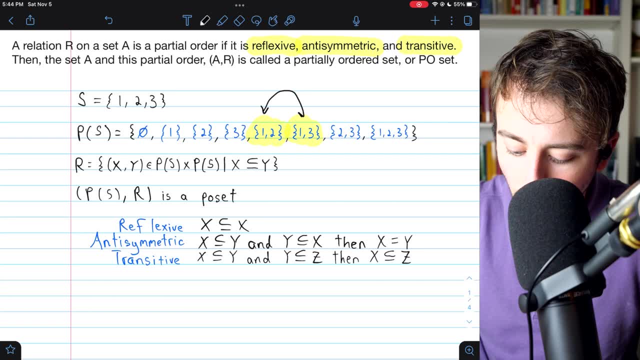 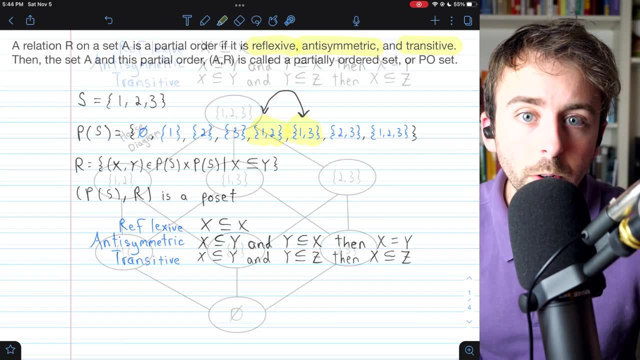 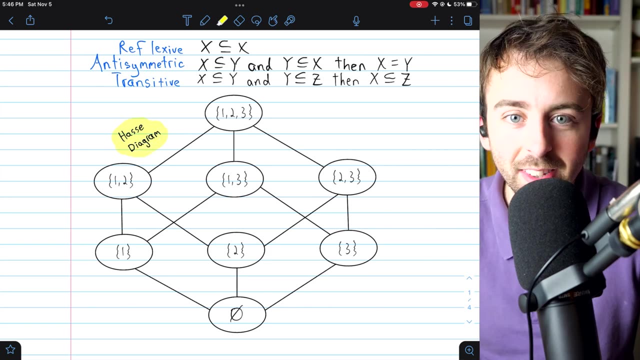 containing 1 and 2, neither of these sets are subsets of each other, So the power set p of s has only been partially ordered. Before we move on to our next example, here is the Haase diagram for this partially ordered set. You may be surprised to see that it doesn't. 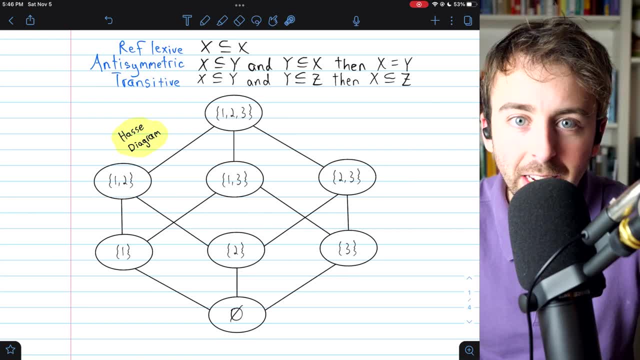 have any arrows indicating the direction of a relation. But that's one of the smart features of a Haase diagram is that it gets around including any arrows. The way it does, that is by ensuring that if there were arrows, they would all be pointing the same direction. 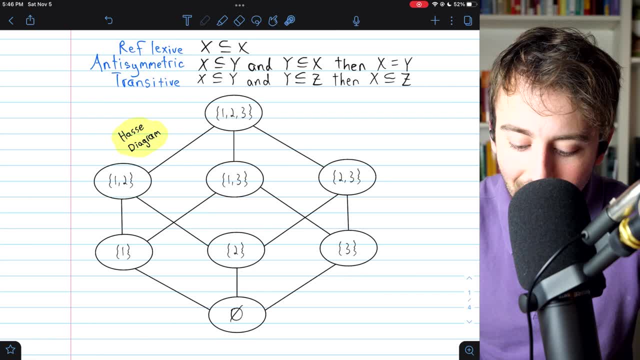 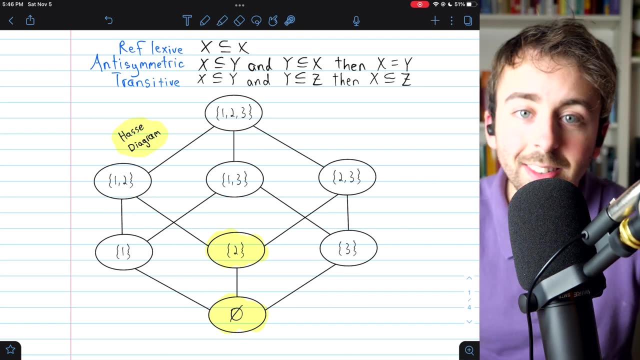 So in fact they're not necessary. In this diagram our relation moves from top to bottom. So, for example, the empty set goes up to the set containing 2.. So I know the direction of this relation. It's that the empty set relates to the set containing 2.. The empty 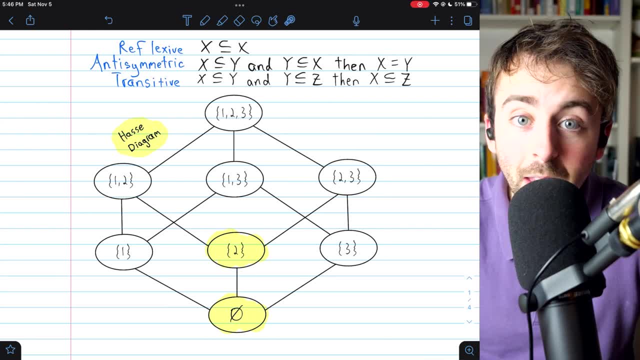 set is a subset of the set containing 2.. Similarly, we go up from the set containing 2 to the set containing 2 and 3.. Thus it's this which is a subset of this, not the other way around. Our relation goes. 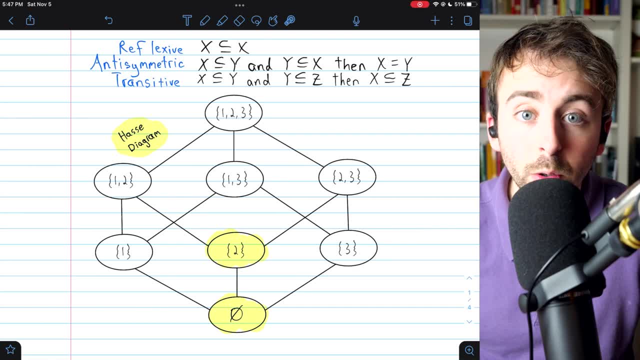 up. You could make a Haase diagram where the relation goes from top to bottom, or left to right, or right to left. Either way, it's great to make sure the relation is always going the same direction, because that allows us to not need arrows. 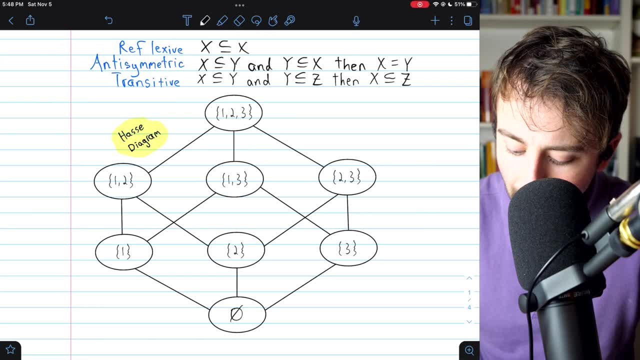 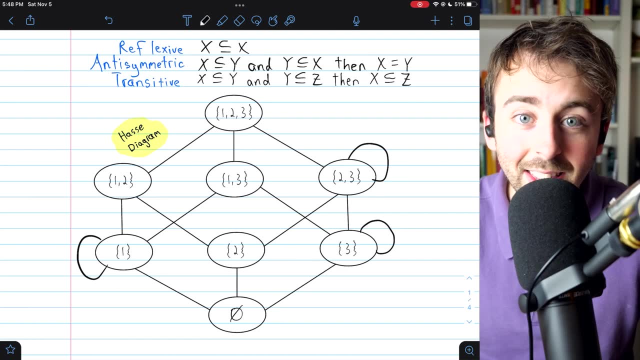 Two other nice features of a Haase diagram. Notice that none of our elements have arrows connecting to themselves. That's because Haase diagrams are 4, representing partially ordered sets, And in a partially ordered set every element always relates to itself, because partial orders are, by definition. 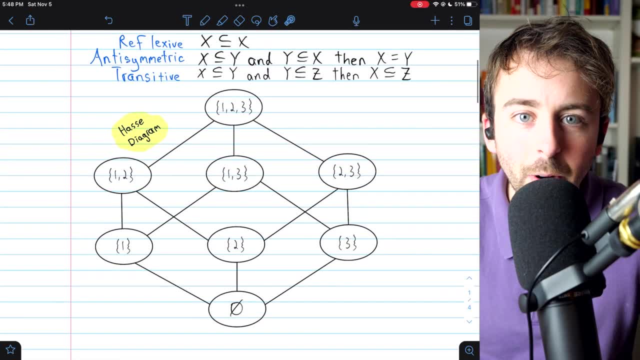 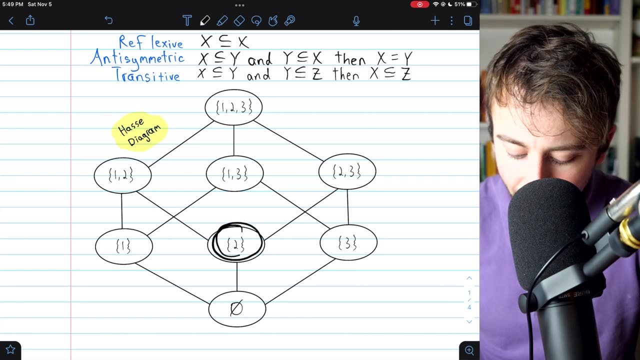 reflexive. So we don't need to clutter up our diagram with arrows indicating those reflexive relations. We know they are there by definition of a partial order. Finally, you may notice that there is no line or arrow joining the set containing 2. 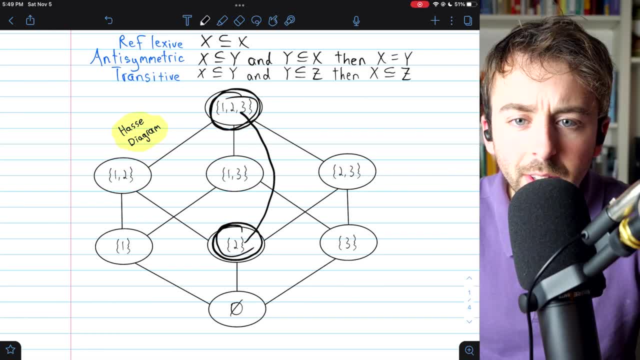 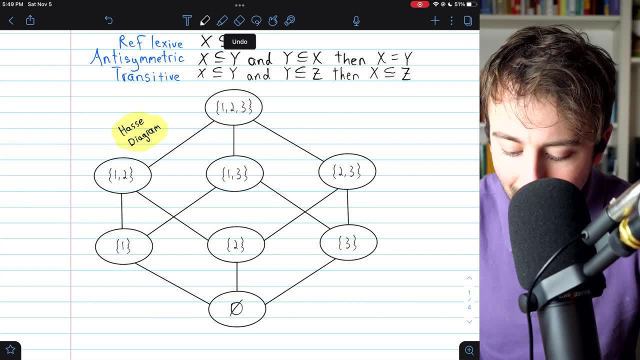 to the set containing 1,, 2, and 3, even though the set containing 2 is a subset of the set containing 1,, 2, and 3.. The reason there's no arrow there is that I know this is a subset. 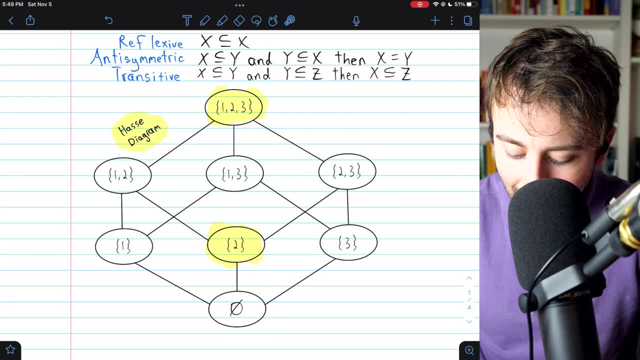 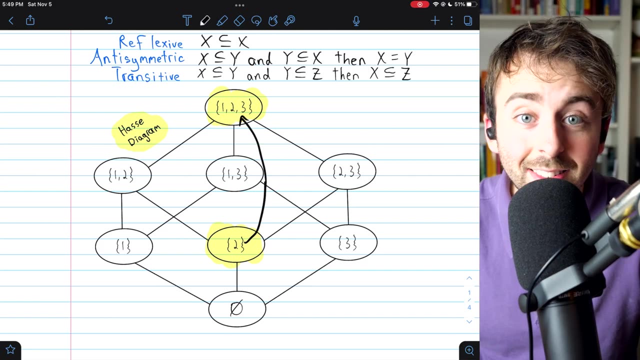 of this by transitivity. Since the set containing 2 is a subset of the set containing 1,, 2, and 3, the relation between these elements is just a result of transitivity And, again, since I know partially ordered sets are transitive, any relation that results from that transitivity. 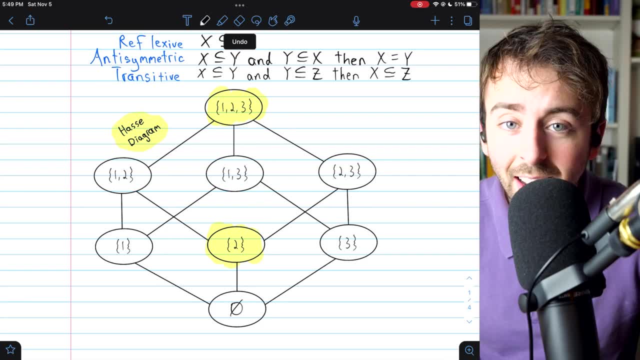 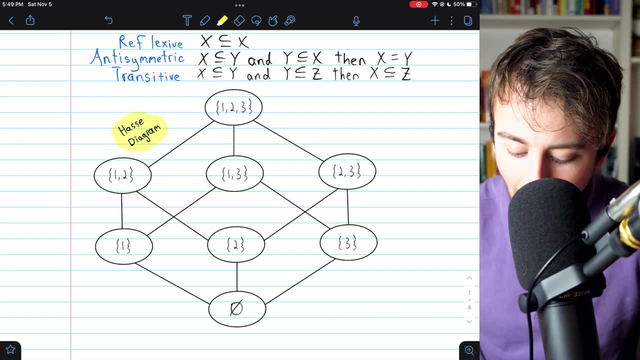 doesn't really need to be represented in the diagram. In the diagram I can see this relation because I know Poe sets are transitive and I see that we can travel along edges from the set containing 2 to the set containing 1,, 2, and 3.. 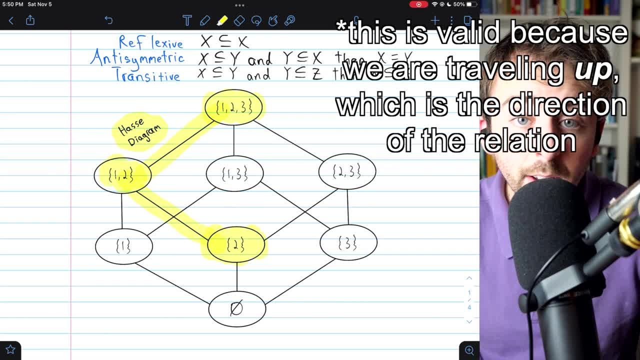 So I can see that we can travel along edges from the set containing 2 to the set containing 1,, 2, and 3.. Since we can travel along edges to get from here to here, I know that this set relates to this one And since we're going up the diagram, I know the direction. 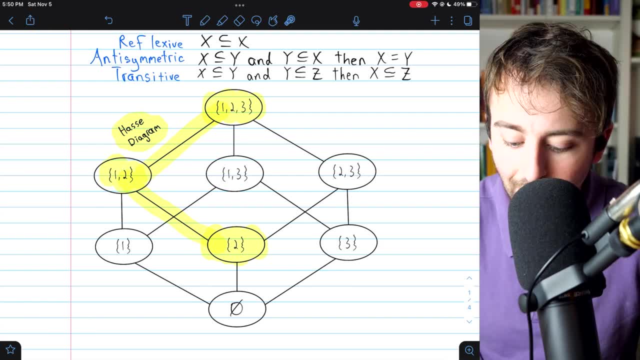 of the relation. The set containing 2 is a subset of the set containing 1,, 2, and 3.. Of course, it shouldn't be surprising that the set containing 1,, 2, and 3 is at the very. 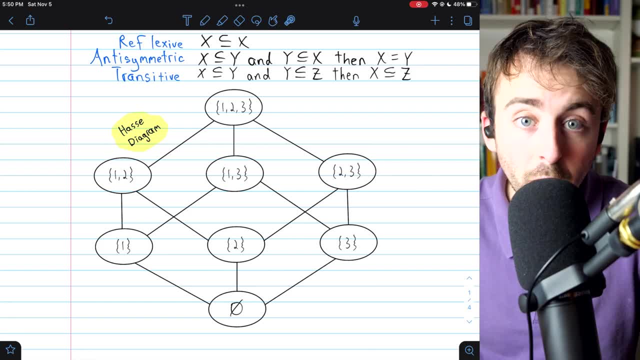 top of the Haase diagram because every element in our partially ordered set relates to the set containing 1,, 2, and 3.. So it's got to be all the way at the top, since I've ordered the elements from bottom to top, And then at the very bottom is the empty set, because 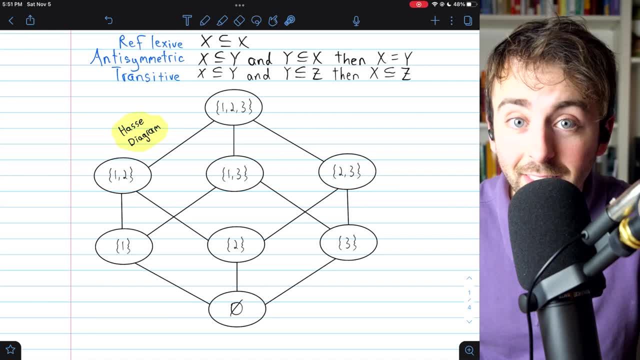 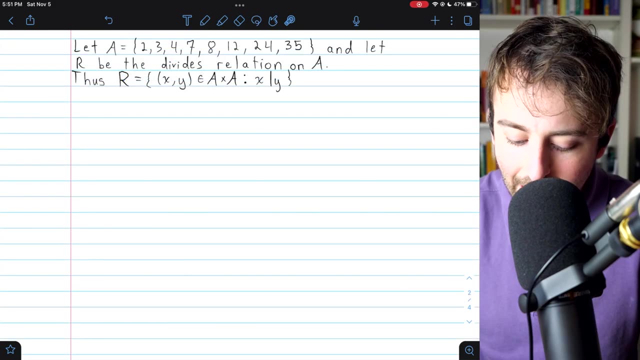 nothing relates to the empty set, since nothing is a subset of the empty set, aside, of course, from itself. Alright, let's go on to one more example, where we'll also define minimal, maximal, minimum and maximum elements. Okay, So this set A be the set containing just a handful of positive integers, And R is going. 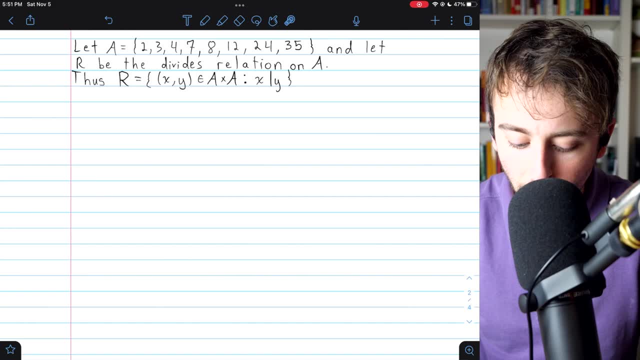 to be. the divides relation on A. So R contains all ordered pairs where X and Y are both from. A and X divides Y, Then this set A along with our divides relation. R forms a poset. Division is reflexive, since every number divides itself. It's also antisymmetric. 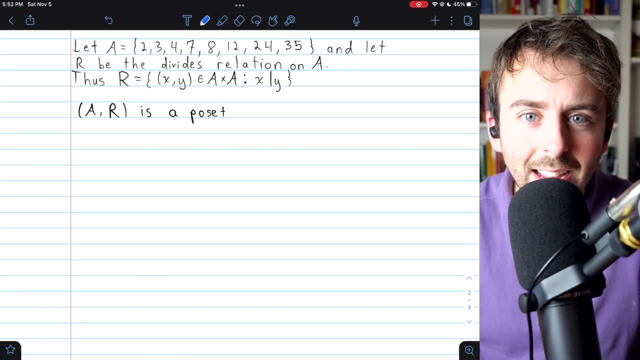 Because if X divides Y and Y divides X, well, the only time that happens is when X equals Y, And certainly division is also transitive. If X goes into Y and Y goes into Z, then X would also have to go into Z. So the divides relation on our set A certainly forms a poset. 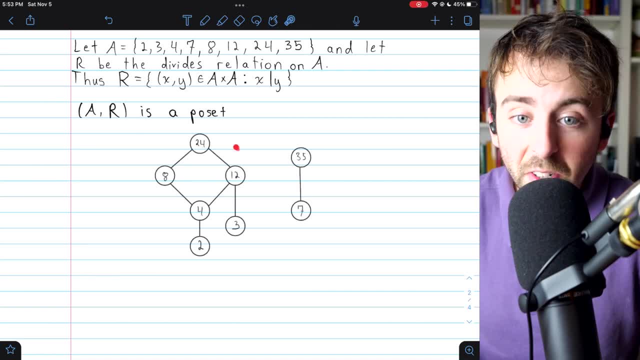 I'll leave it to you to verify those rules more formally. Here is the Haase diagram for the poset. Again, this diagram is ordered from: R. So R is going to be the divisor of R. So R is going to be the divisor of R So R is going to be the divisor of R So R is going to be. 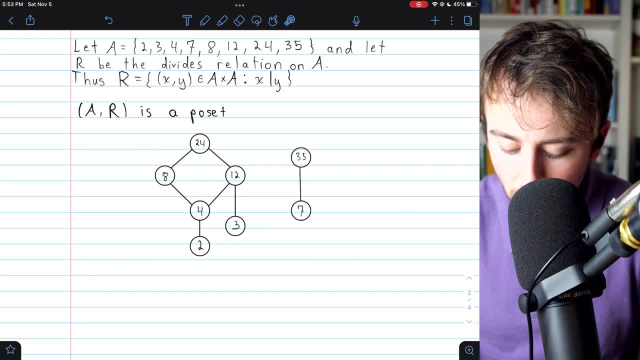 from bottom to top, So we can go up from 2 to 4.. That means that 2 divides 4.. Notice how I can travel across edges to get from 2 to 24, which tells me that 2 divides 24.. 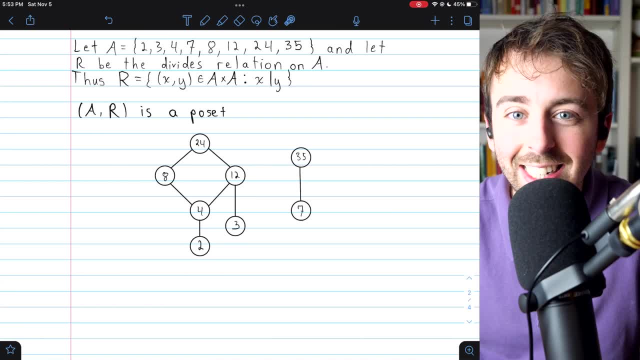 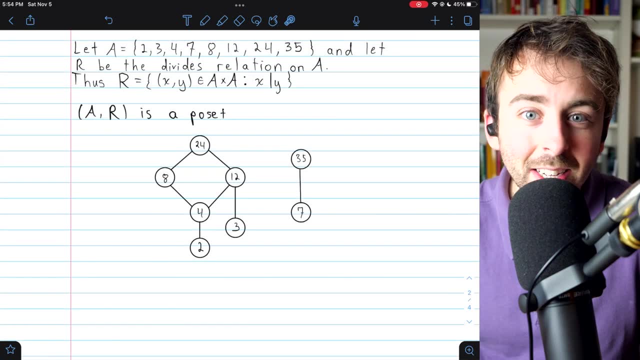 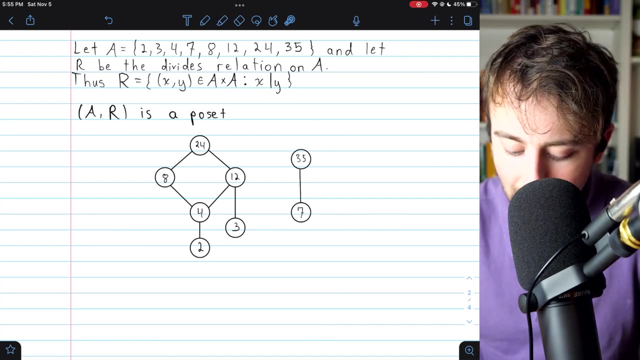 Again, every element divides itself, So we don't really need to draw those arrows in. That's part of what makes a Haase diagram so elegant. And notice again, that has not been completely ordered. Not every pair of elements have a relation to each other. There's no way to get between 3 and 4 by moving up the diagram. They 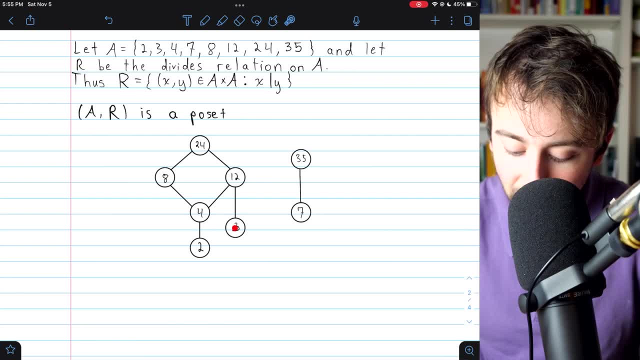 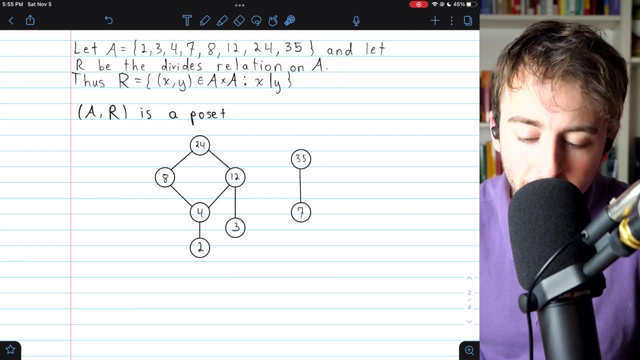 don't relate to each other in any way. Remember you've got to move up the diagram because that's the direction the relation takes in this diagram, from bottom to top. 7 and 35,. they don't relate to any of the numbers over here, which is interesting. This Haase diagram has two. 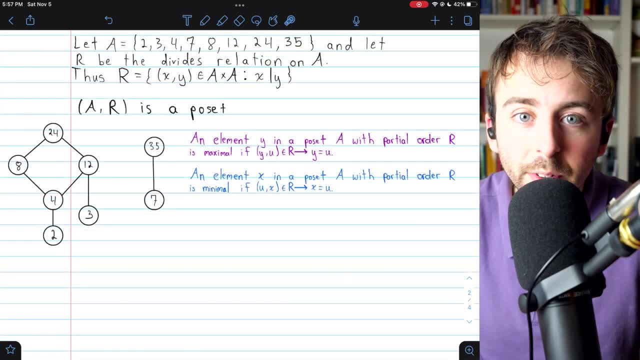 disconnected components. And this leads to a few quick definitions. We say an element y in a partially ordered set, A is maximal if y relates to no element except itself. So if y relates to u, then y must equal u. In our Haase diagram we can find the maximal elements at the tops of 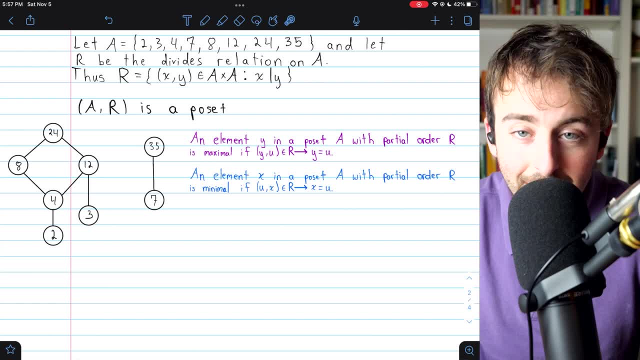 the components. 24 is a maximal element. It doesn't relate to anything except itself, So it's all the way at the top of its component. Similarly, 35 is a maximal element. It doesn't relate to anything except itself. Notice, of course, maximal elements are not unique. 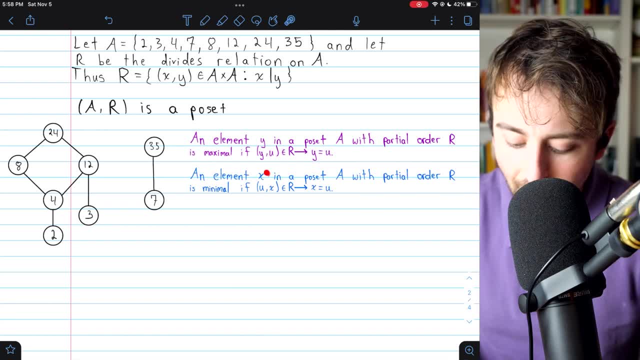 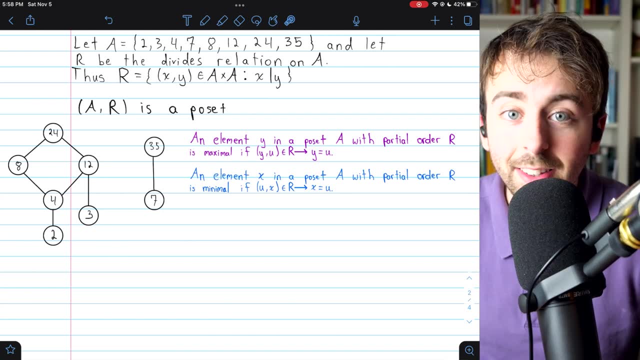 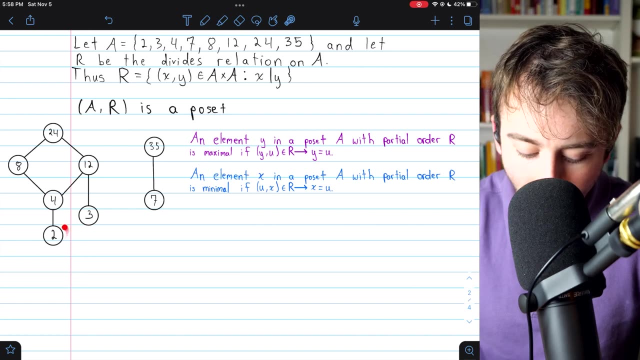 The definition of minimal element is similar. We would say an element x is minimal if the only thing that relates to x is x itself. So if u relates to x, x must equal u. These, of course, can be found at the bottom of the diagram. So if y relates to x, then y must equal u. 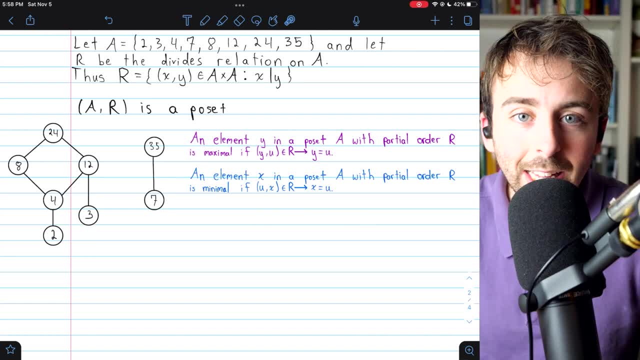 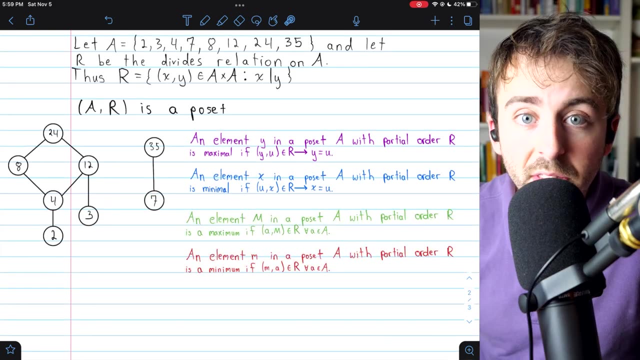 of the components, 2 is a minimal element because nothing relates to 2 except for itself in this set. Similarly, 3 is a minimal element. Nothing relates to 3 here except for itself, And 7,, of course, is also minimal. There are then the similar but certainly different ideas. 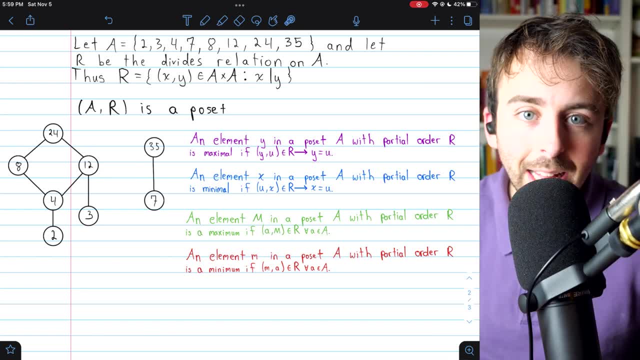 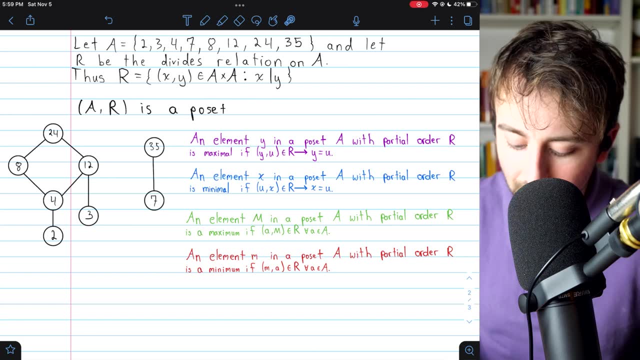 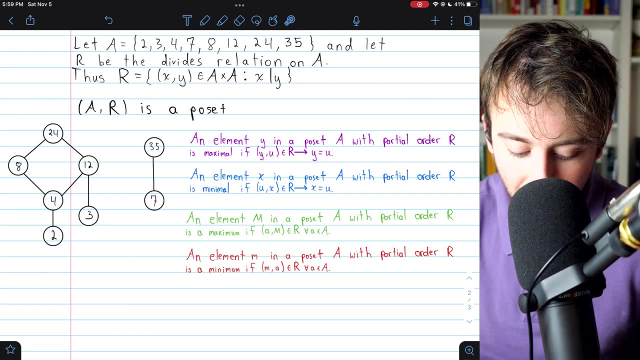 of a maximum element and a minimum element. We would say that an element in a partially ordered set is a maximum if x is x itself. So if y relates to x, x must equal u, And if y relates to x, x must equal u. And similarly we would say that an element little m is the minimum of a partially 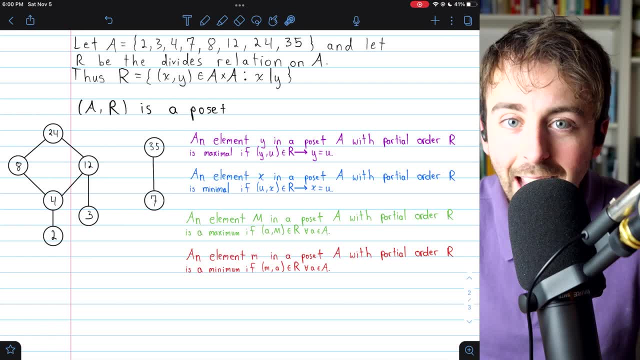 ordered set. So if y relates to x, x must equal u, And similarly we would say that an element little m is the minimum of a partially ordered set. If it relates to everything else, Again, there's no minimums here. 2 does not relate to everything. 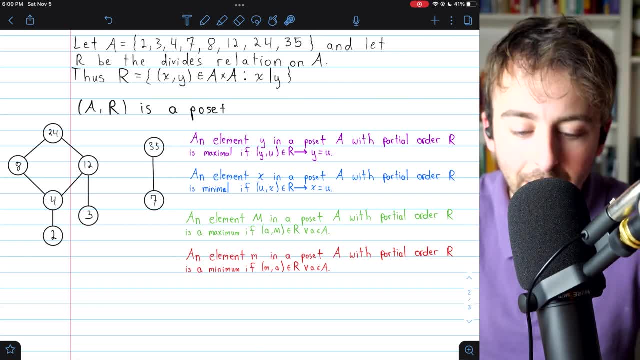 since it doesn't relate to 3,, 7, or 35.. And 3 doesn't relate to everything, since it doesn't relate to 4,, 2,, 8,, 7, or 35. So there are no minimums here. This is in contrast to our first. 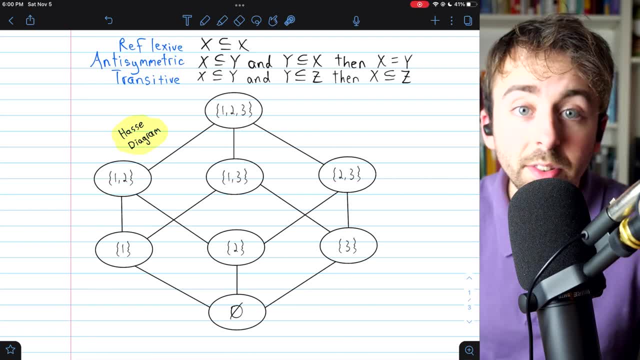 example. In our first example the empty set was a minimal element. It's at the bottom of its component. So if y relates to x, x must equal u, And similarly we would say that an element little m is the minimum of a partially ordered set. 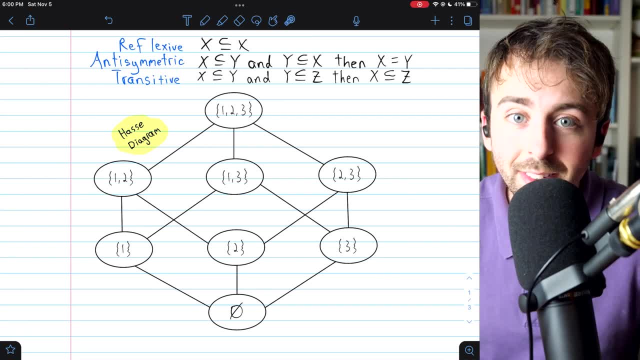 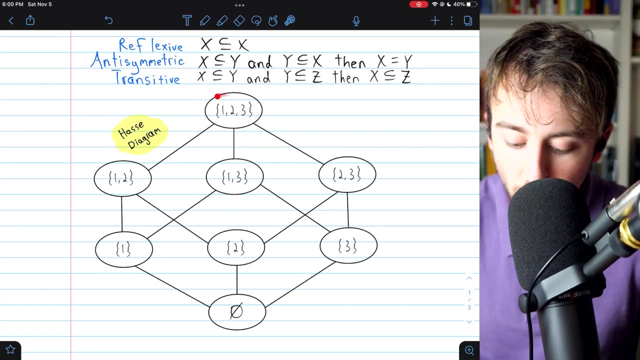 But it is also minimum. It relates to every single element in the partially ordered set. The original set S- the one containing 1,, 2, and 3, is also maximal. It's at the top of its component And it's maximum. Everything relates to this set. This set is the maximum of the partially ordered. 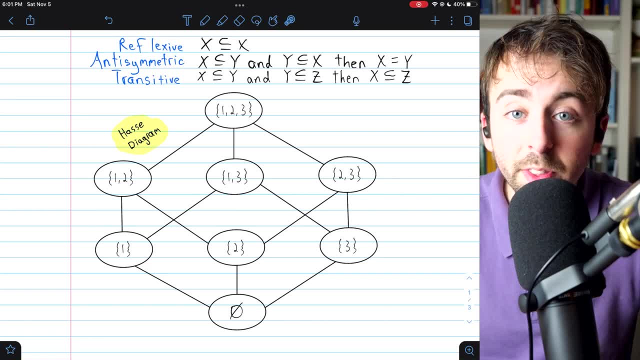 set it belongs to. If there is a minimum or if there is a maximum, those will be unique in a partially ordered set. If there is a minimum or if there is a maximum, those will be unique in a partially ordered set. 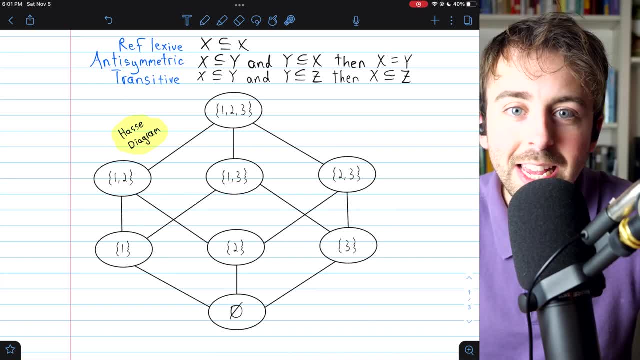 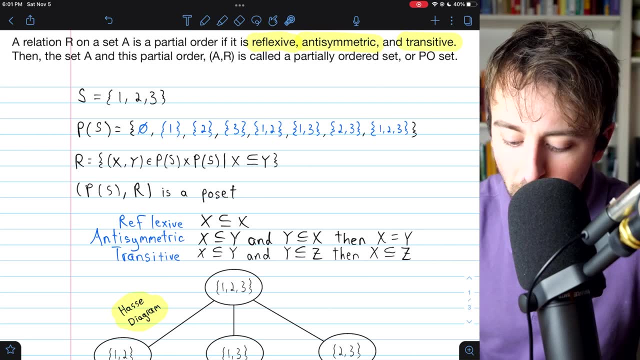 If there is a minimum or if there is a maximum, those will be unique in a partially ordered set, Which is a straightforward proof I'll leave to you. Let me know if you want any help in the comments. But that's it for this intro to partially ordered sets and Haase diagrams. Hope it was helpful. Here's just a quick review. 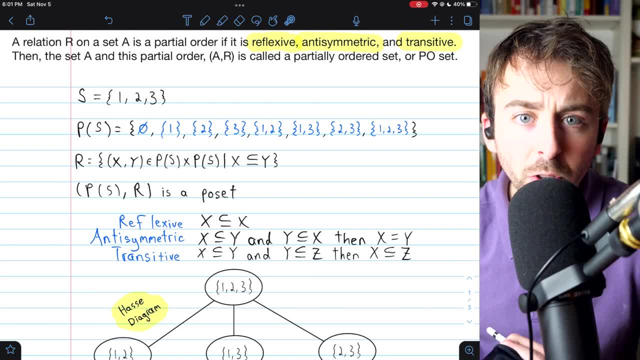 We say that a relation R on a set A is a partial order. if it's reflexive, anti-symmetric and transitive, Then the set A, along with that partial order, makes a partially ordered set. We call it a partial order because it's not necessary that every pair of elements 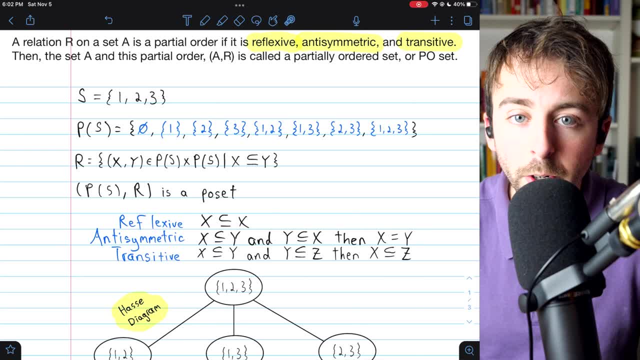 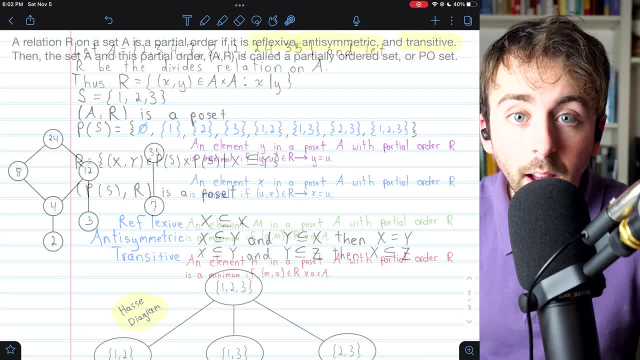 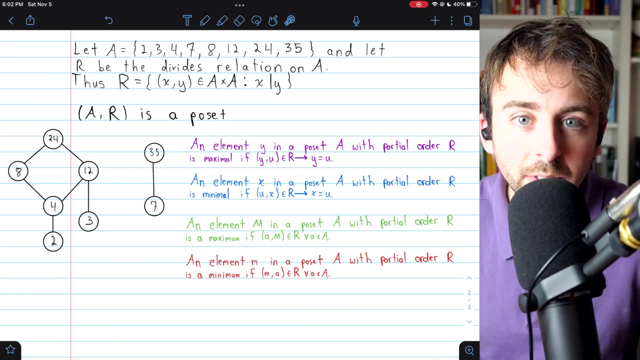 in a Poe set are put in any particular order. You could have some elements, like we said, this one and this one- that just do not relate to each other in any way. A Haase diagram is a way of representing a partially ordered set that uses the features of a Poe set to cut back on the clutter. 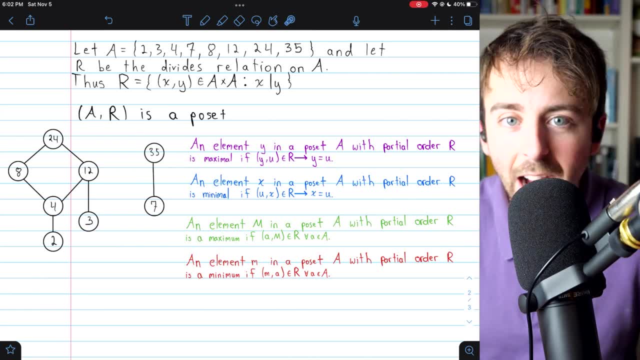 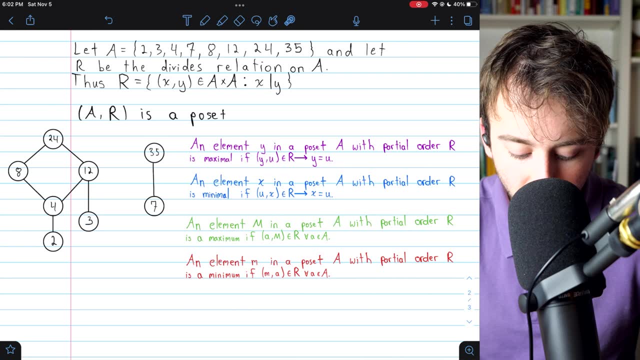 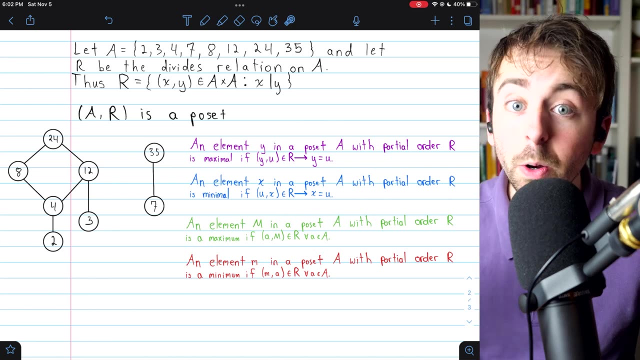 of the diagram. In a Haase diagram, there are no arrows representing the reflexive relationships between an element and itself, because we know they exist. Same thing with transitive relations: There are no arrows representing the transitive relations And in fact we don't need arrows explicitly to indicate direction, because Haase diagrams are created.